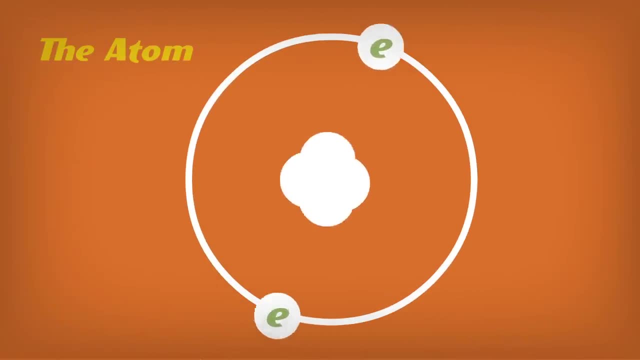 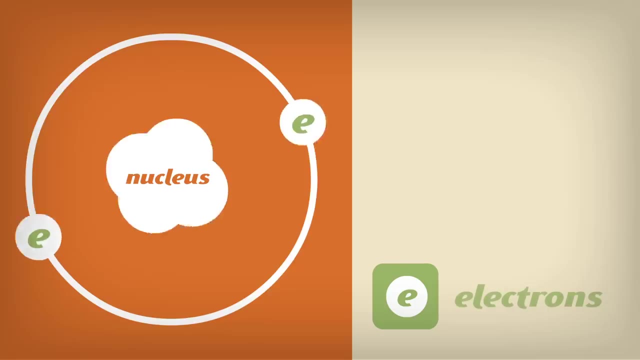 But the atom is not the smallest unit of matter. Experiments found that each atom has a tiny, dense nucleus surrounded by a cloud of even tinier electrons. The electron is, as far as we know, one of the fundamental, indivisible building blocks of the universe. 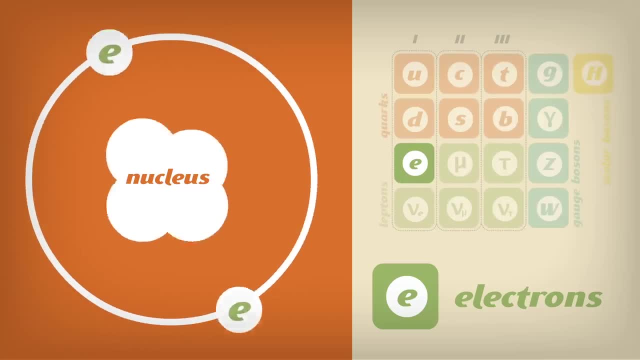 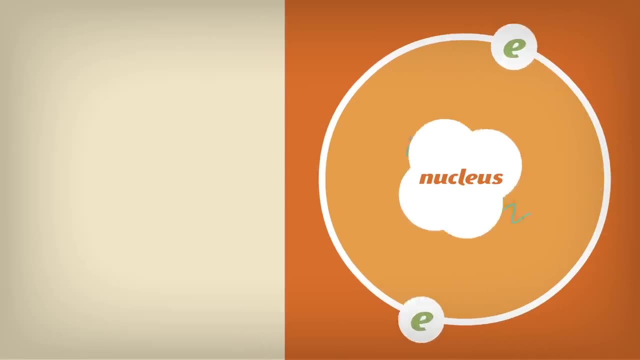 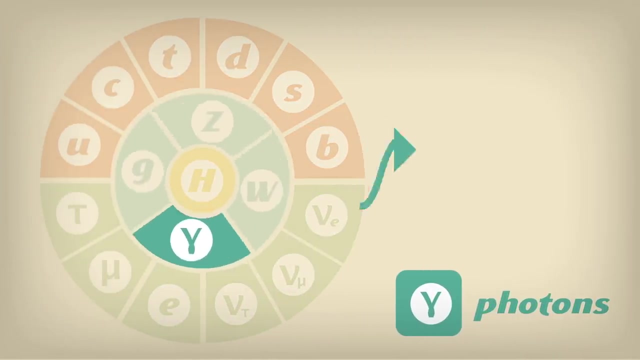 It was the first Standard Model particle ever discovered. Electrons are bound to an atom's nucleus by electromagnetism. They attract each other by exchanging particles called photons, which are quanta of light that carry the electromagnetic force, one of the fundamental forces of the Standard Model. 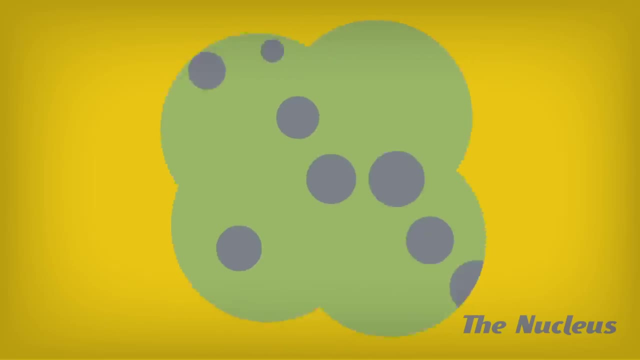 The nucleus has more secrets to reveal, as it contains protons and neutrons, Though once thought to be fundamental particles on their own, in 1968, physicists found that protons and neutrons are actually neutrons, but they are actually made of quarks. 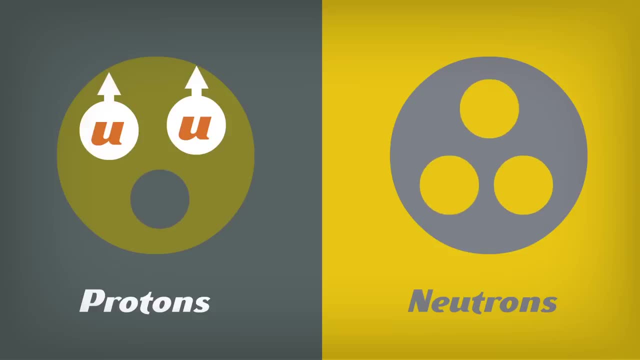 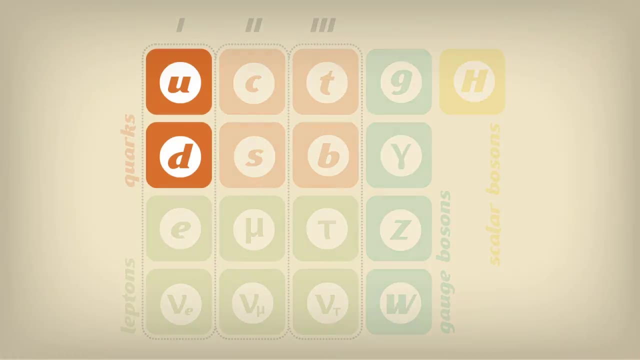 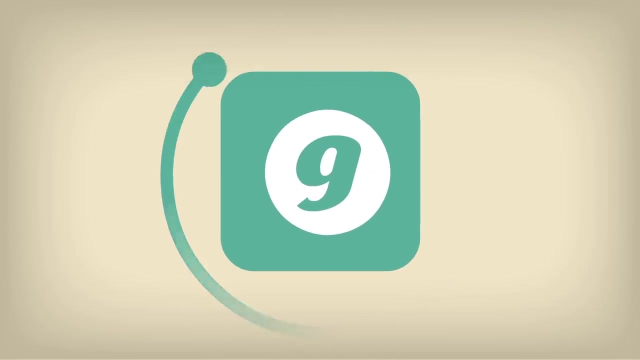 which are indivisible. A proton contains two up quarks and one down quark. A neutron contains two down quarks and one up. The nucleus is held together by the strong force, another fundamental force of the Standard Model, Just as photons carry the electromagnetic force. 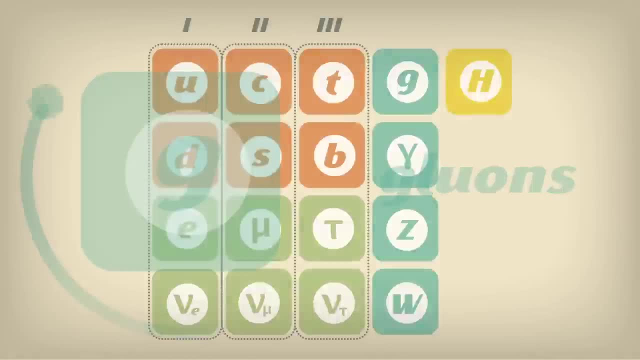 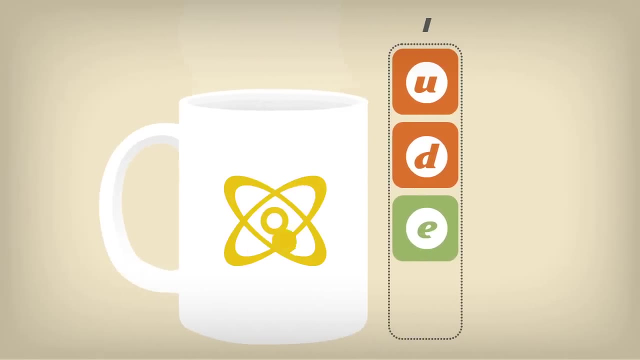 particles called gluons carry the strong force Electrons, together with up and down quarks, seem to be all we need to build atoms and therefore describe normal matter. However, high-energy experiments reveal that there are actually six quarks. 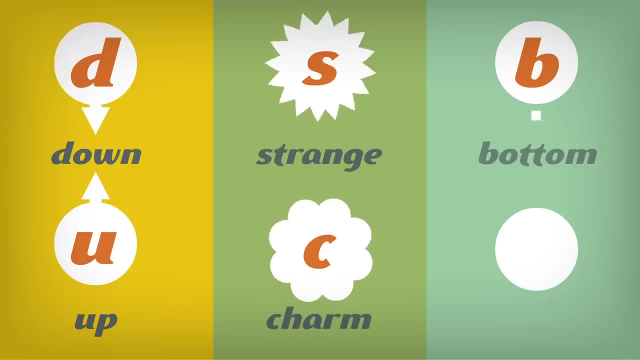 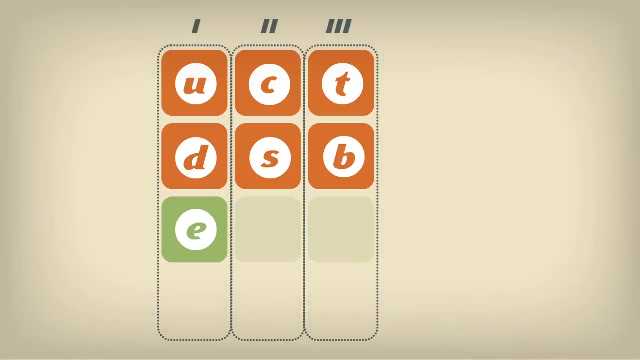 down and up, strange and charm, and bottom and top, And they come in a wide range of masses. The same was found for electrons which have heavier siblings called the muon and the tau. Why are there three, and only three, different versions? 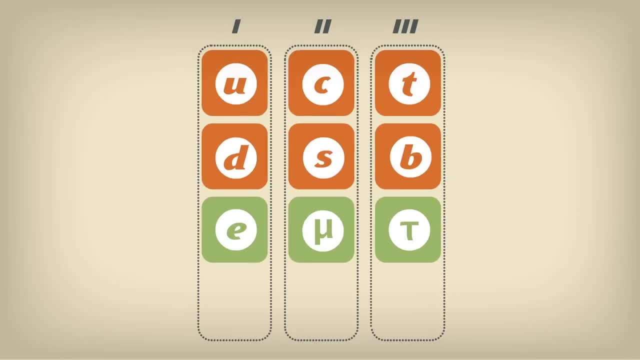 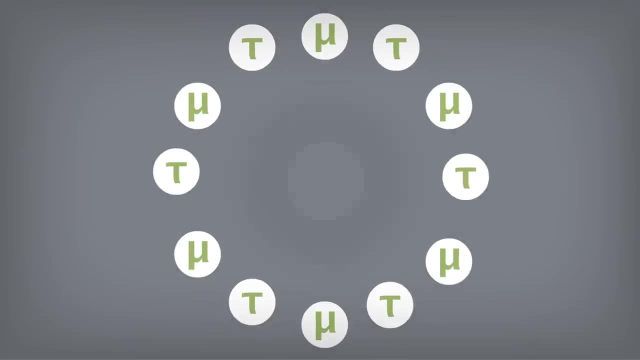 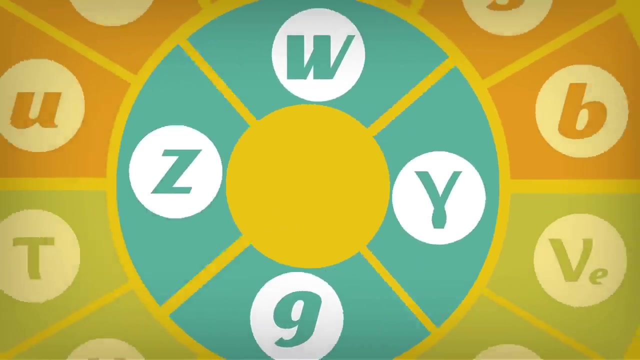 of each of these particles. This remains a mystery. These heavy particles are only produced for very brief moments in high-energy collisions and are not seen in everyday life. This is because they decay very quickly into the lighter particles. Such decays involve the exchange of force-carrying particles. 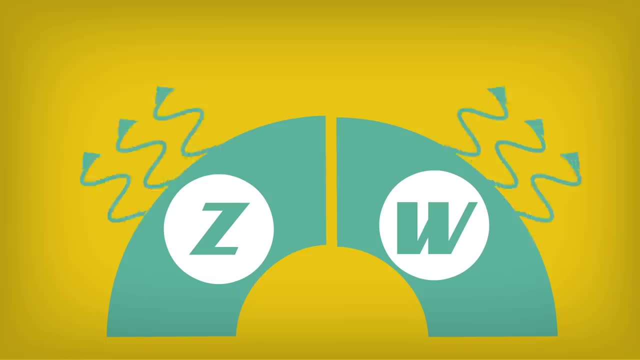 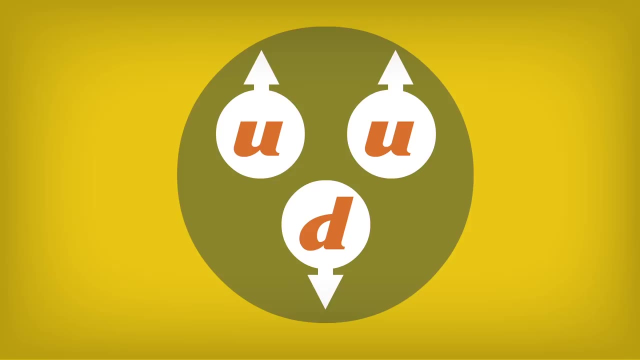 called the W and Z which, unlike the photon, have mass. They carry the weak force, the final force of the Standard Model. This same force allows protons and neutrons to transform into each other, a vital part of the fusion interaction.